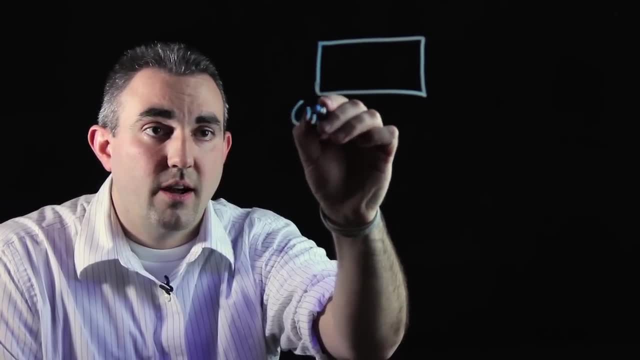 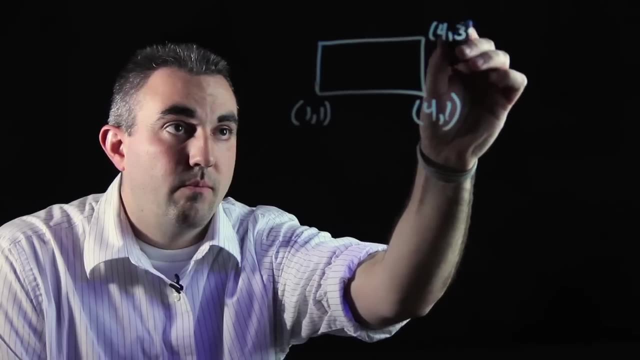 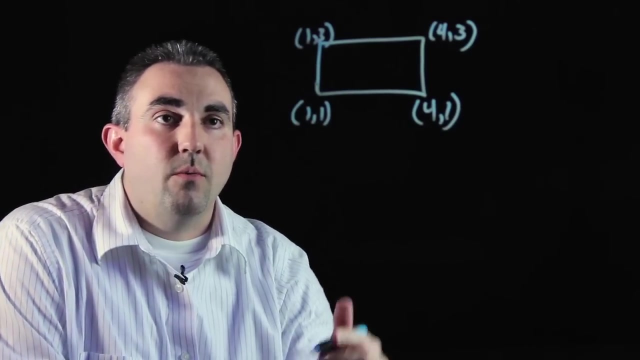 was on a coordinate plane with points, So we're going to call this one comma one, four comma one. This will be four, three, And up here will be one comma three. The first thing you want to remember is what a diagonal is. A diagonal is a line that cuts straight across. 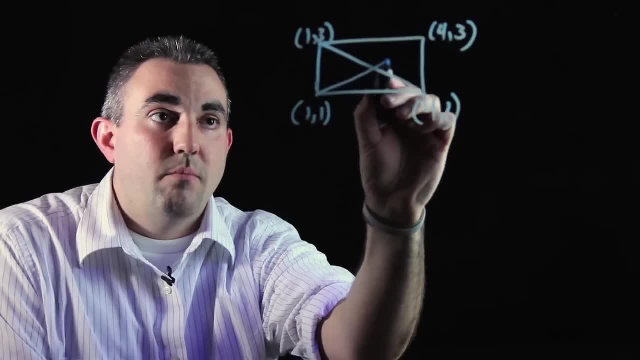 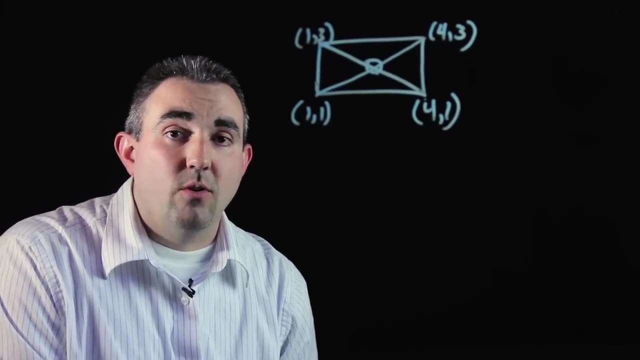 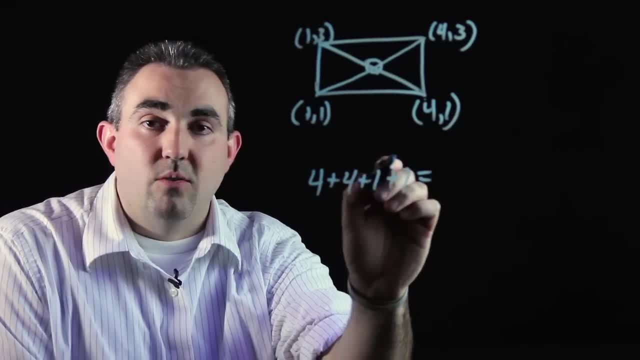 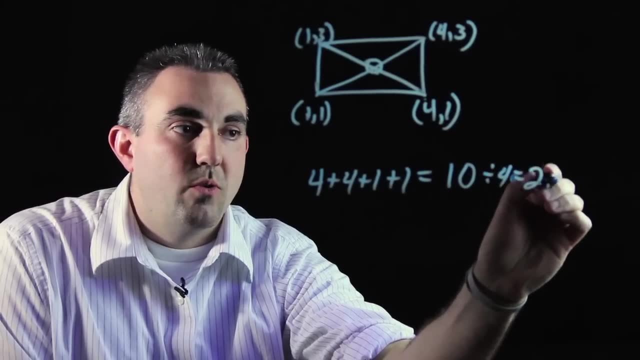 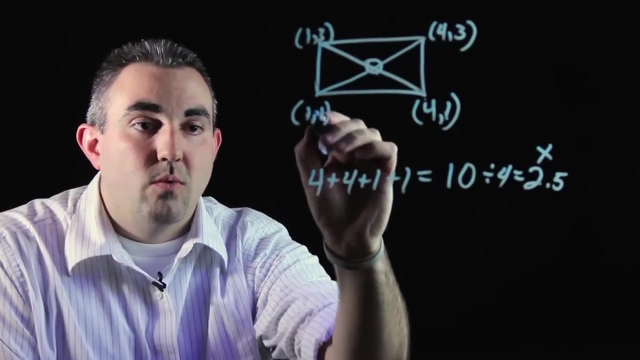 4 plus 4 is 8, plus 1 plus 1, 2 more gives you 10.. Take that answer and divide it by 4 and you get 2.5 for your x. Now you want to do the same thing with all your y coordinates: 3 plus 3 plus 1 plus 1.. 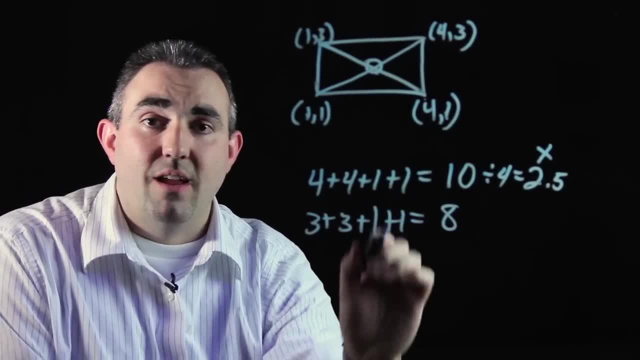 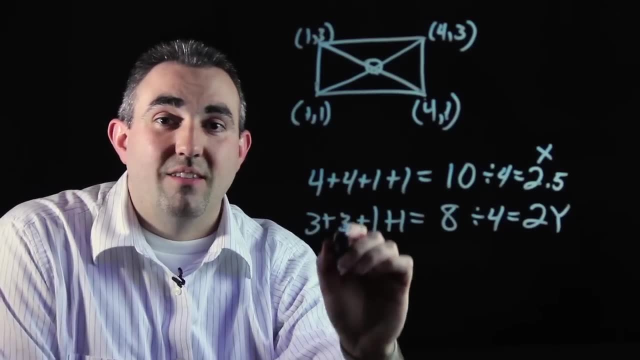 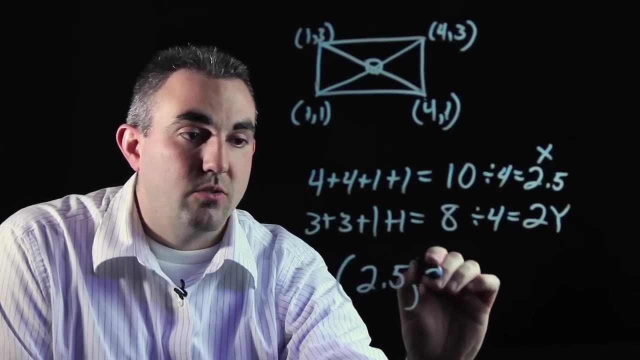 That's 6 plus 1 is 7 plus 1 is 8.. You want to take that number and divide it by 4.. That gives you 2.. This is your new y number, So our centroid will be located at x point 2.5 and y point being 2.. 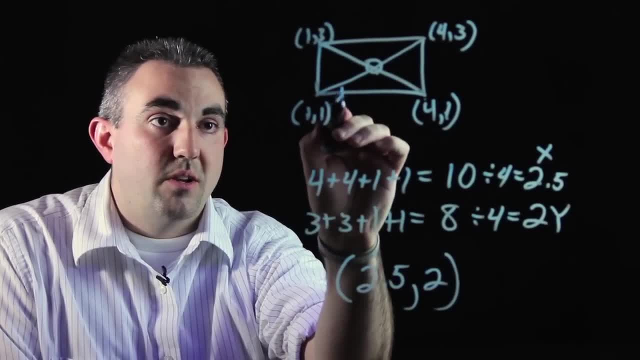 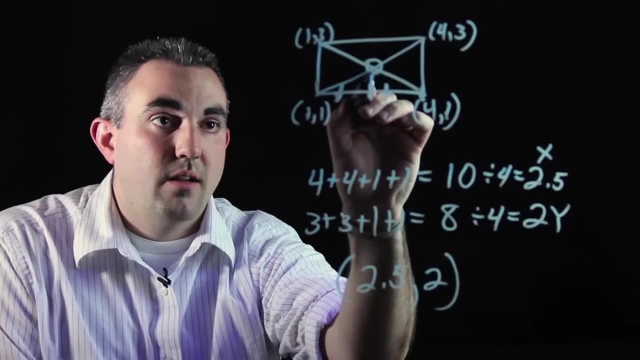 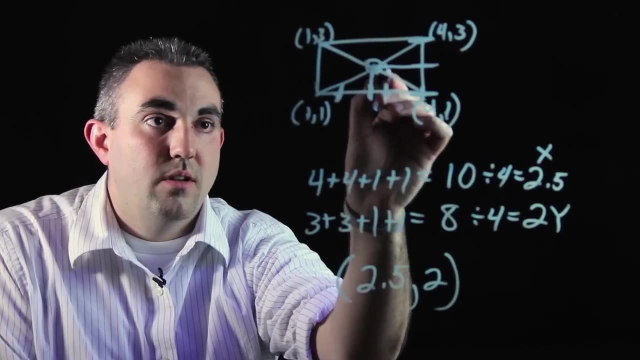 So, if this is 1 and this is 4,, this would be 2,, this would be 3, this would be 4,. 2.5 is somewhere right in between 2 and 3.. And if this is 1,, 2,, 3,, here's 2,, here's 2.5. 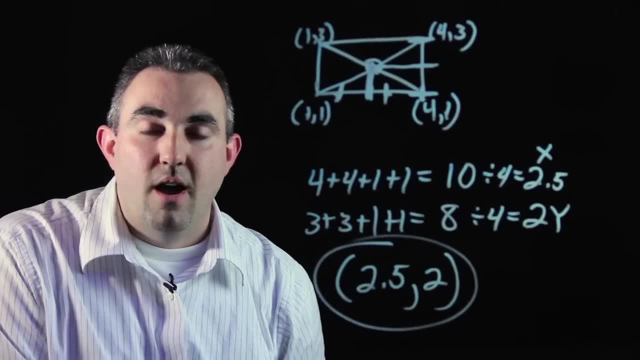 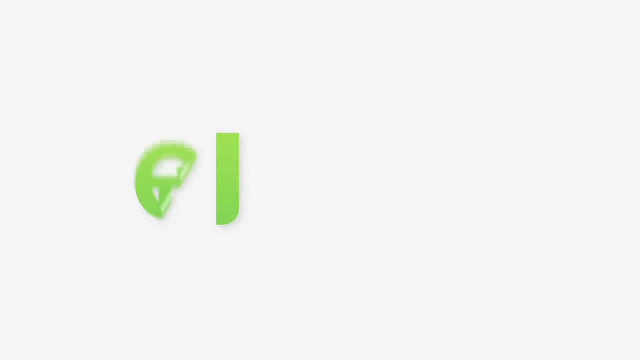 And that's 2.5.. That's where our centroid is 2.5 comma 2.. I'm Tom Ruiz. You do the math.